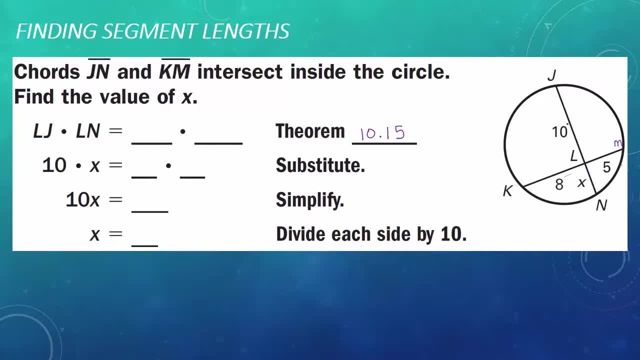 which says that if I have two chords intersecting inside a circle, then the product L J times L N is equal to L K times L M. So I have 10 times X is equal to L K, which is 8 times L M, which is 5.. 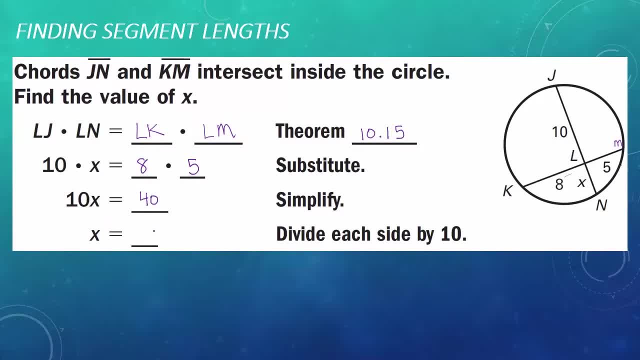 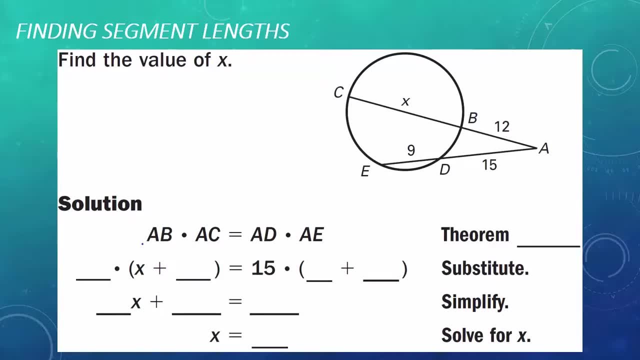 8 times 5 is 40. Isolate X by dividing both sides by 10.. X is equal to 4.. So I'm going to use Theorem 10.16 to solve for the value of X. Example 2 is another one for finding segment lengths. 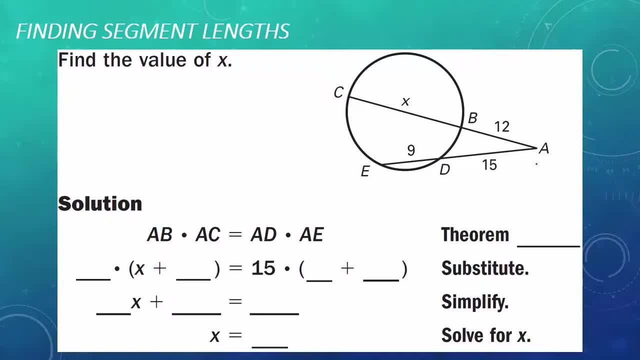 This time I have two secants intersect at the same point And for this I need to find the value of X. So I'm going to be using Theorem 10.16 to solve for the value of X In 10.16,. I know that the length of AB times the entire secant. 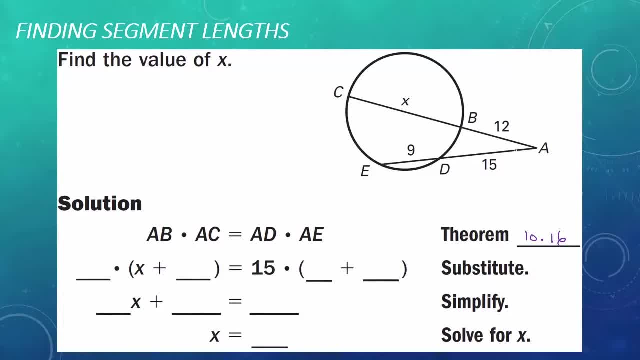 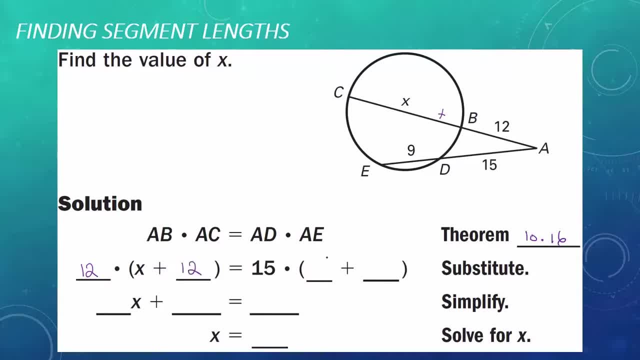 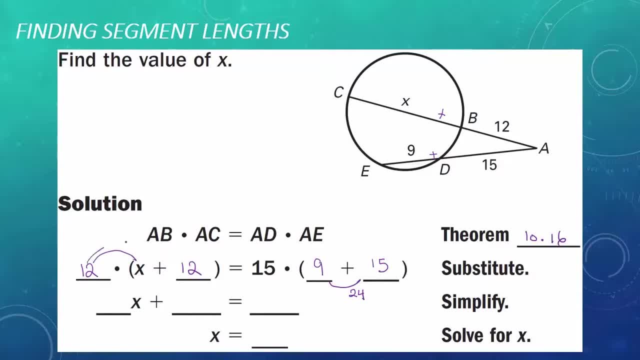 Solve for X. We start off by distributing the 12 with X and positive 12.. 12 times X is 12.. 12 times 12 is 144.. 15 times 24 is 360.. Subtract 144 on both sides and you get that 12X is equal to 216. 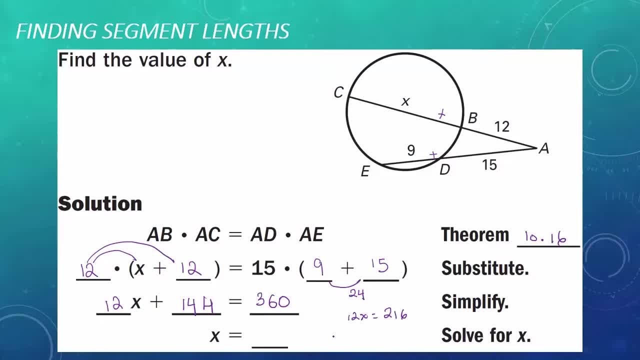 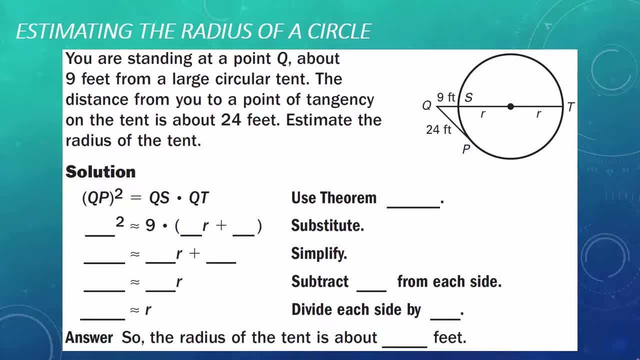 Divide both sides by 12.. And 216 divided by 12 gives us X equals 18.. Example 3, estimating the radius of a circle. You are standing at a point Q, about 9 feet from a large circular tent. The distance from you to a point of tangency on the tent is about 24 feet. 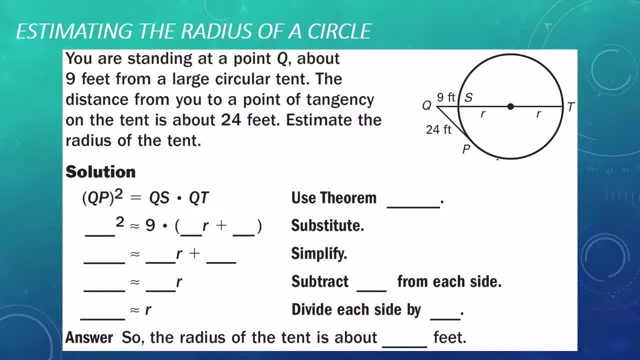 Estimate the radius of the tent In this circular tent and our point of tangency. we have a tangent and we have a secant, So I'm going to use theorem 10.17 to solve for our radius. According to 10.17, our tangent squared, QP squared, is equal to the external part of our secant, which is QS. 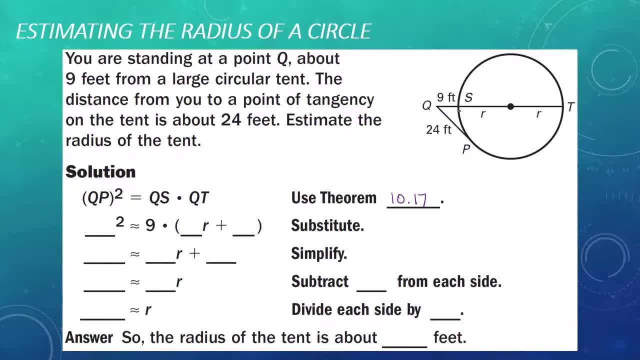 times the entire length of our secant, which is QT. We know that QP is 24, so that's going to be 24. squared is approximately equal to 9,, which is my external length of my secant, so QS. 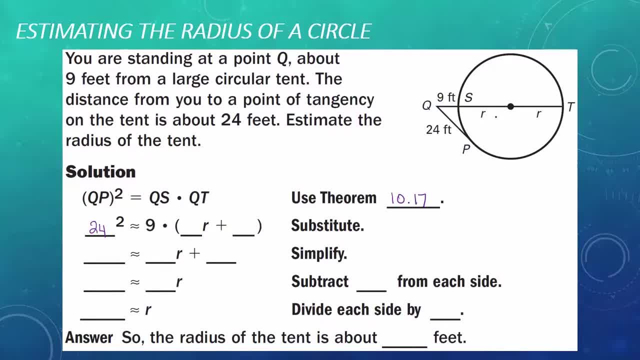 times the entire length over here. so it'll be 9 plus R plus R. We know R plus R is going to be 2R, so it's 2R plus 9.. 24 squared is 24.. That's 576.. 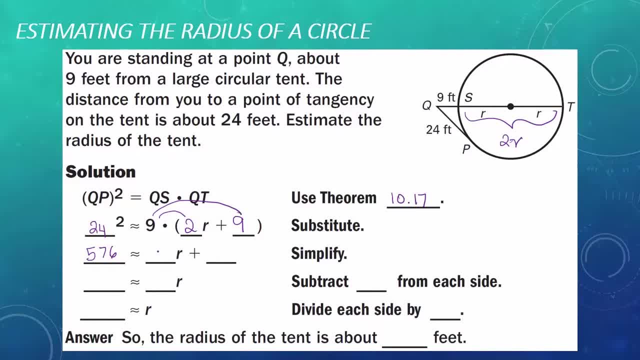 Distribute the 9 to get rid of the parentheses: 9 times 2R is 18R. 9 times 9 is 81.. Subtract 81 on both sides, 576 minus 81 is 495.. It's approximately equal to 18R. 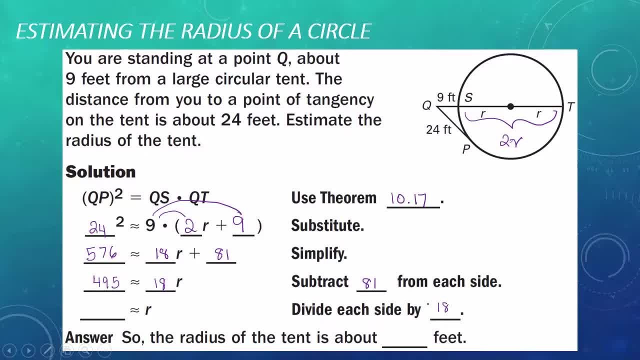 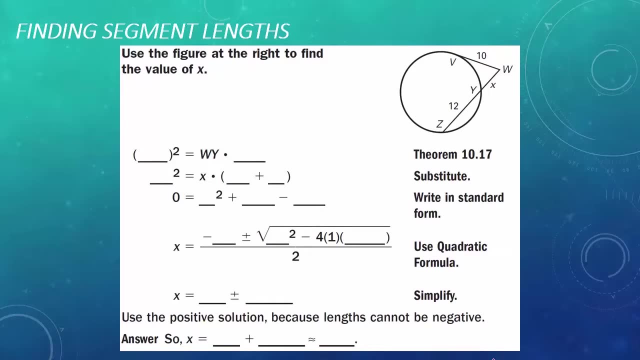 Divide both sides by 18, and 495 divided by 18 gives us approximately 27.5.. So our radius for the tent is about 27.5 feet. Example 4.. Again another one finding segment lengths. This time I have a tangent and I have a secant meeting at the same point outside the circle. 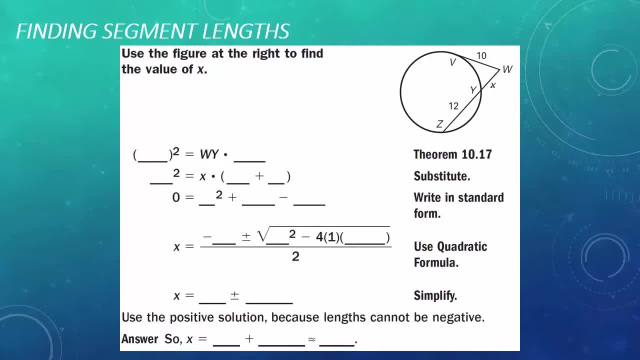 According to Theorem 10.17,, we're going to take the square of our tangent, which is VW, and that is equal to the external length of our secant, which is WY times the entire length of our secant, which is WZ. 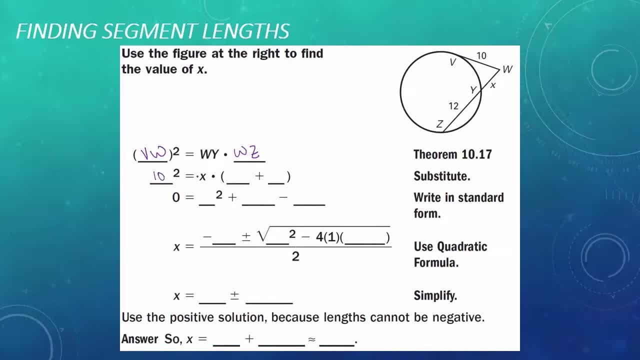 We know that VW is 10, so it's going to be 10 squared. and we know that WY is X and the entire length of WZ is X plus 12.. When we multiply this out, you're going to end up with: 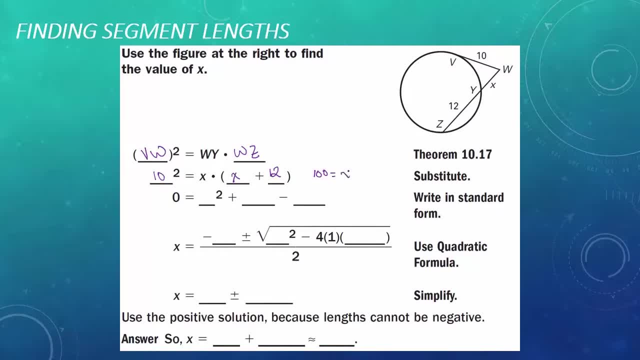 10 squared, which is 100, is equal to X times X, which is X squared plus 12X. This is a quadratic function. In order to solve this, you need to write it in standard form, which means: subtract 100 on both sides. 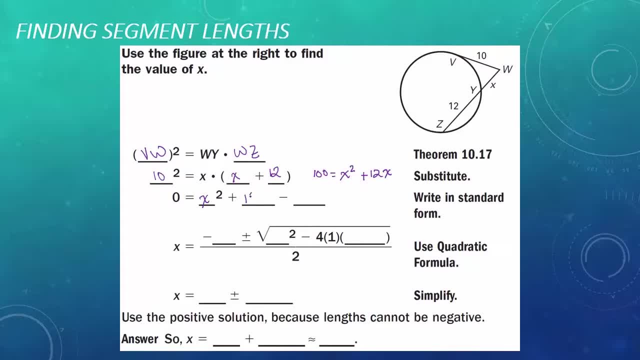 What you end up with is X squared plus 12X minus 100 is equal to 0.. From here, use the quadratic formula to solve for X. Remember the quadratic formula is negative: B plus or minus the square root of B squared minus 4AC. 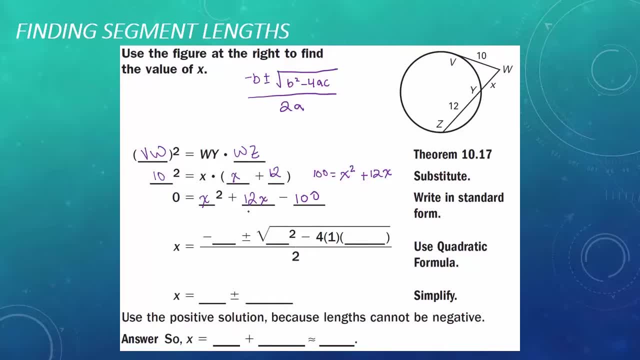 all divided by 2A. In this case, my B is 12, so it's going to be negative. 12 plus or minus 12, squared minus 4 times 1 times negative 100, all divided by 2.. Going to do the math over here. 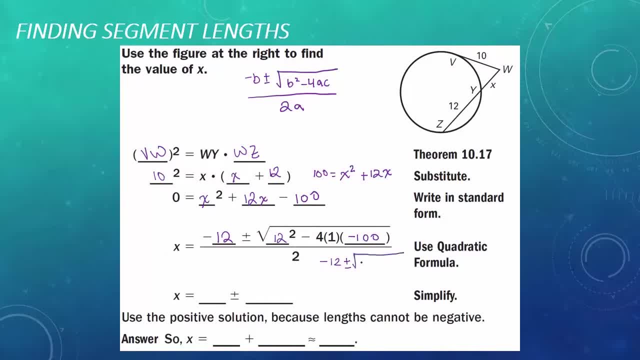 This is negative. 12 plus or minus 12 squared is 144.. Negative 4 times 1 is negative, 4.. Negative 4 times negative: 100 is positive 4.. All divided by 2.. This becomes negative 12 plus or minus the square root of 544 divided by 2.. 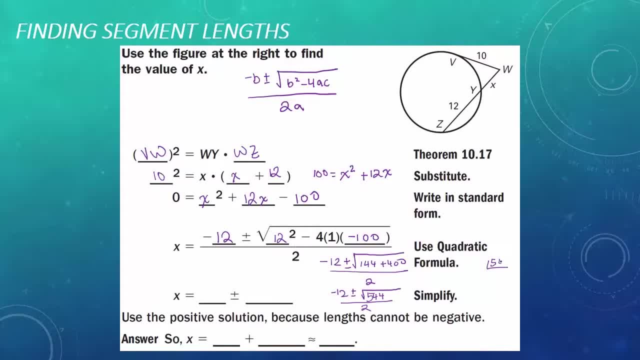 Simplify the square root of 544.. So the smallest prime number I can divide 544 by is 2.. That gives me 272.. Divide that again by 2.. That gives me 136.. Divide again by 2. That gives me 68.. 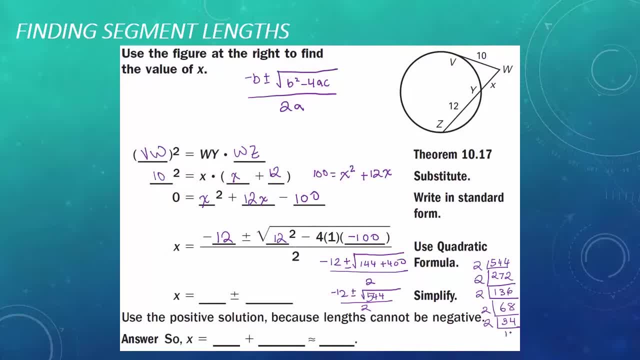 2 gives me 34.. 2 gives me 17.. And the next number I can divide 17 by is 17.. Every time I have a pair, I'm going to take one of those guys out. Get rid of the other. 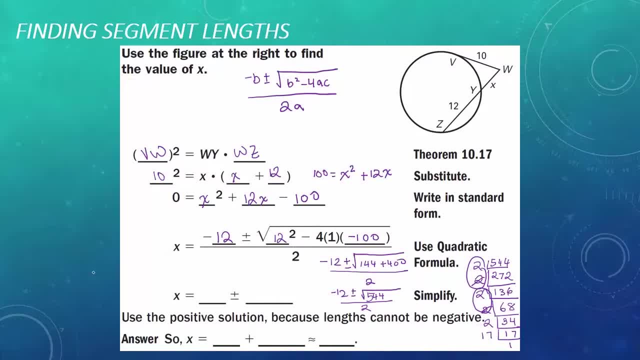 Take one of those guys out, Get rid of the other. Whoever is left goes back in the house, So I'm going to put the work over here. This simplifies down to negative 12 plus or minus 4 times the square root of 34 divided by 2.. 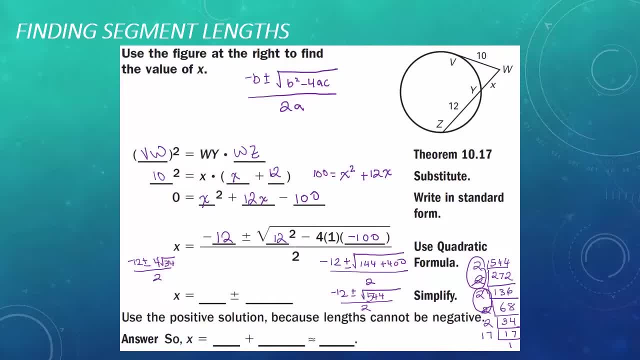 I can simplify both negative 12 and the plus or minus 34.. Essentially, I can rewrite this as negative 12 divided by 2, plus or minus 4, square root of 34 divided by 2.. Negative 12 divided by 2 gives me negative 6.. 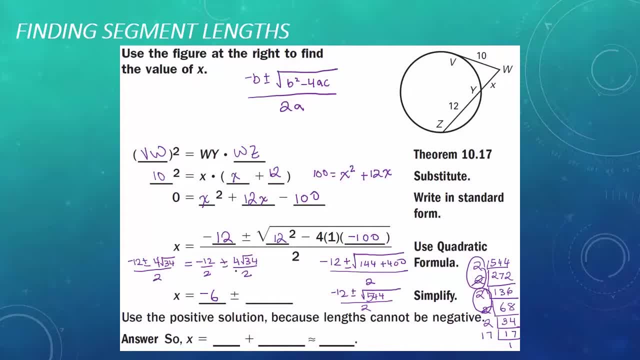 Plus or minus 4 square root of 34 divided by 2.. I can simplify the 4 and 2.. 4 divided by 2 is 2.. So that's 2 square root of 34.. And so x is the positive value of negative 6 plus 2 square root of 34, because what we're looking for 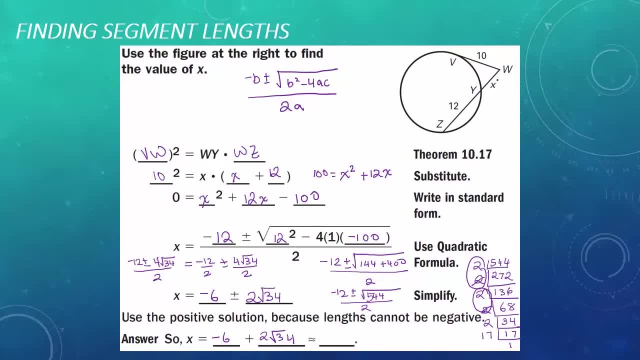 which is x is a length, and you can never have a negative length. You can plug this into your calculator. So negative 6 plus 2 square root of 34 is just going to be 5.66.. Alternatively, you could have just taken this value over here. 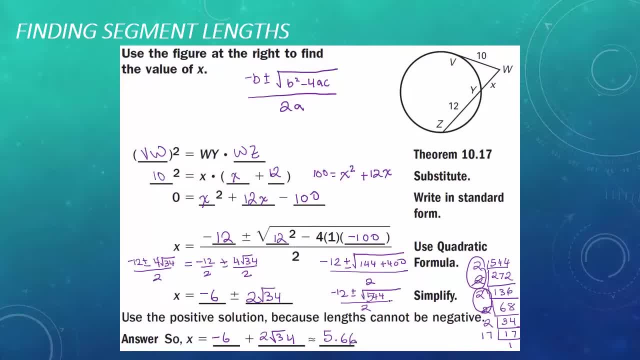 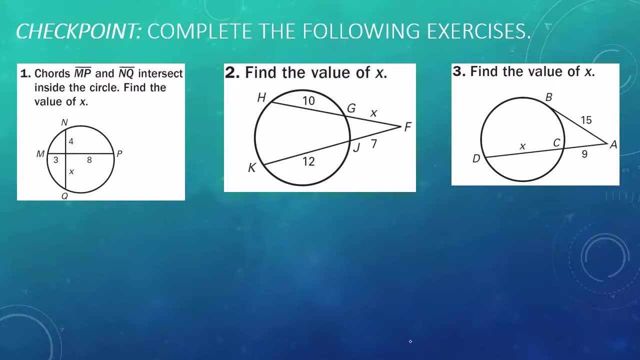 Negative 12 plus or minus square root of 544 divided by 2.. Plug the positive function into your calculator and, given the decimal answer as your solution, Checkpoint problem number 1, 2, and 3 are yours. In checkpoint problem number 1, chords of line segment MP and line segment NQ intersect inside the circle.